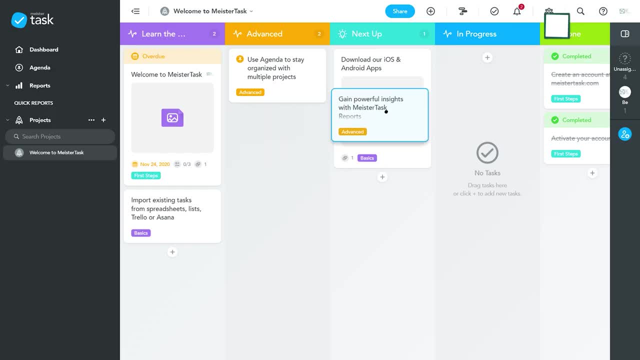 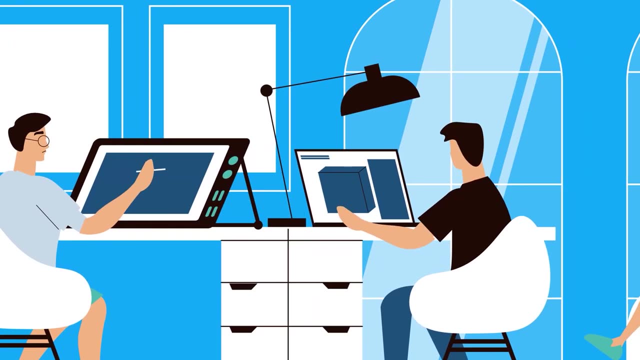 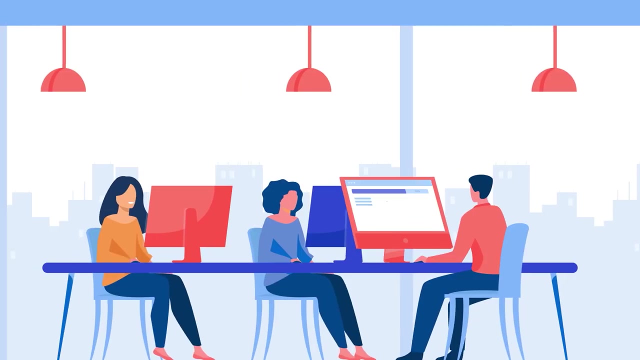 your productivity. we've compiled a list of the 7 best task management softwares, So, without any further ado, let's jump right into the video. Looking for an animation studio that can turn your story or idea into animated visuals, Look no further than 10Studio. Our team of experts creates animated explainer videos that 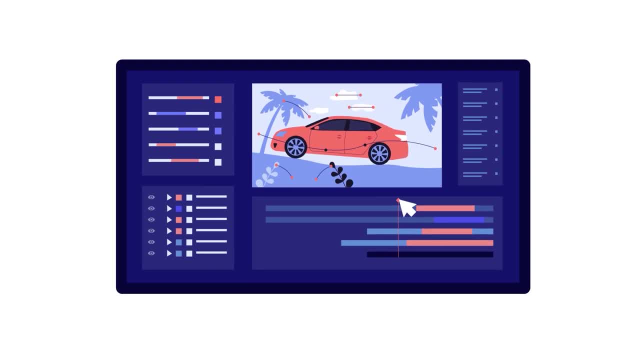 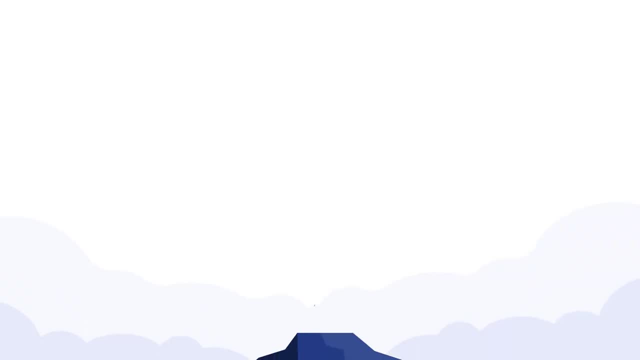 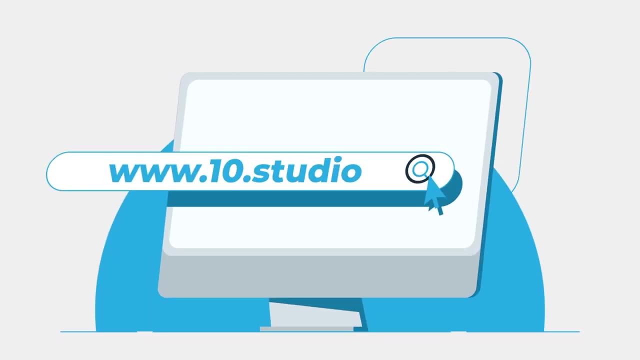 simplify complex ideas and bring your message to life. Our experience can help you tell your story in a way that engages your target audience and makes them remember it. Don't miss out on this opportunity to stand out from your competition. Visit our website to know more at www.10.studio. 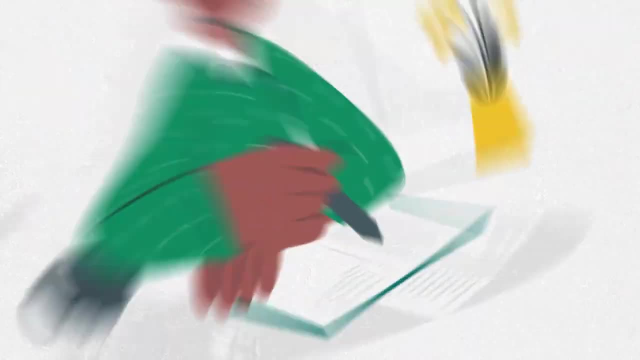 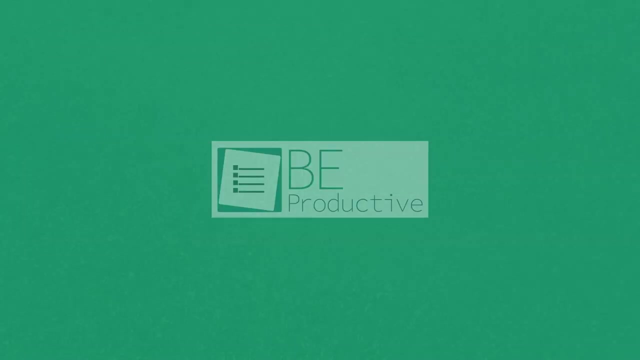 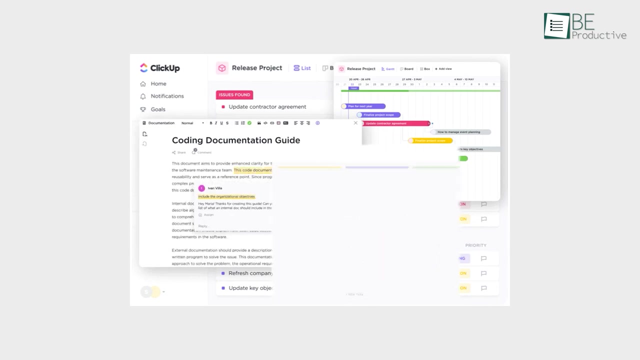 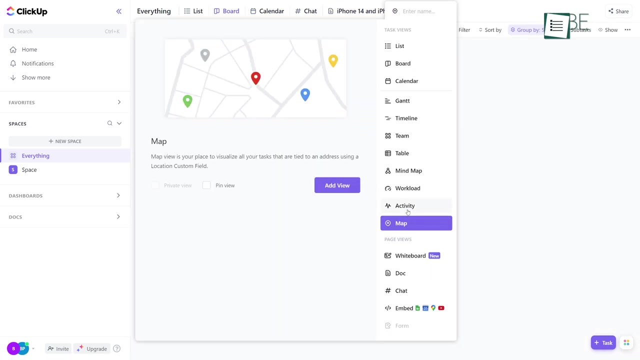 First on the list, we have ClickUp, which offers a comprehensive task management system that streamlines your workflow and boosts your productivity, bringing all your tasks, docs, chats and goals into one place, With its robust set of features and tools. 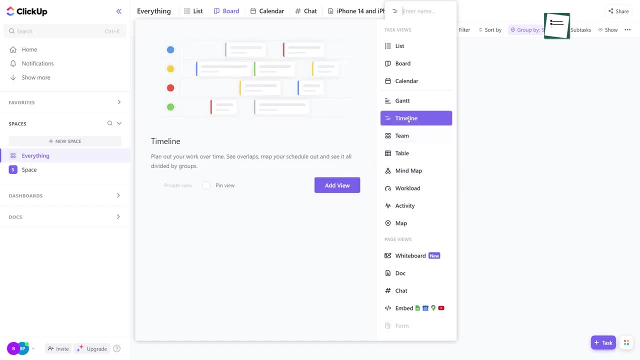 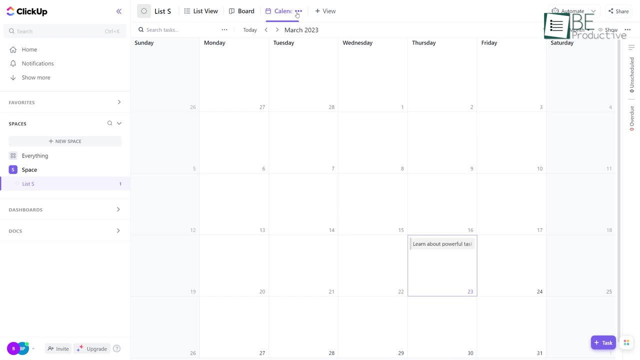 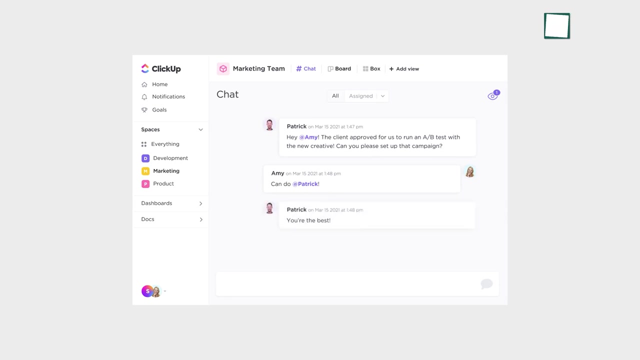 ClickUp helps you track, manage and complete your tasks faster and more efficiently than before. With customizable task views, you can choose from list, board or calendar views and tailor the columns to suit your needs. However, it simplifies communication among team members, making collaboration easier. 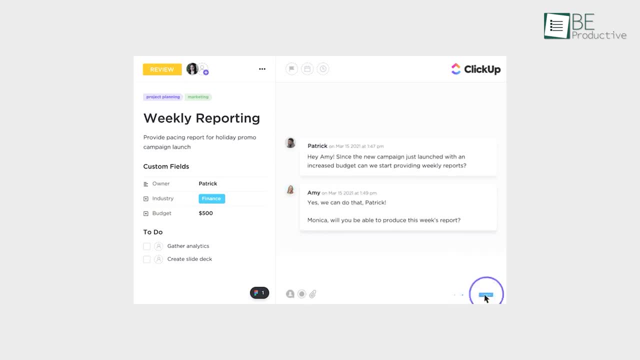 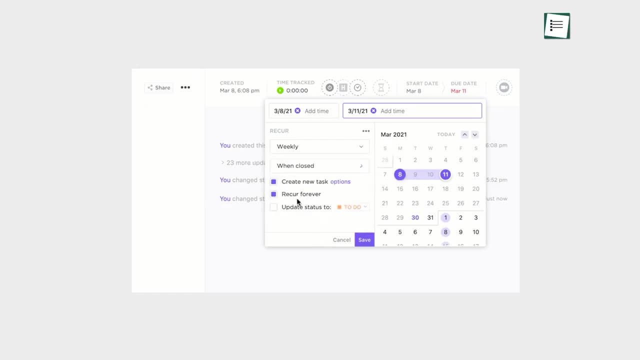 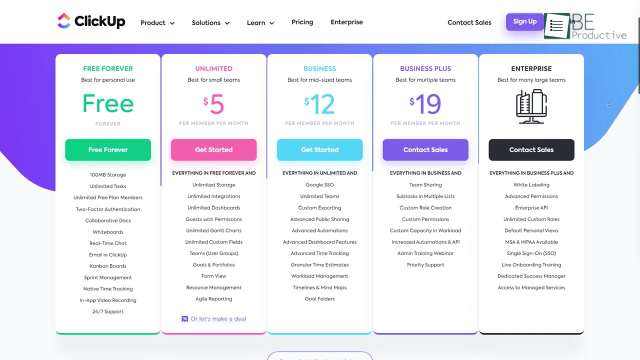 Moreover, you can generate customizable or pre-designed reports and can also share information securely. It also helps you to manage time by allowing you to create schedules, track time, organize calendars and more. What makes it even more understanding is that you can access all of its amazing features for free. 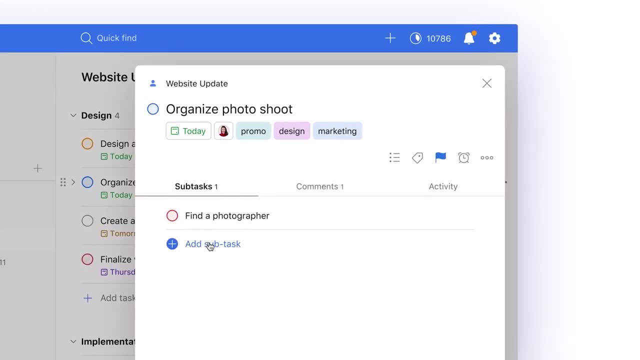 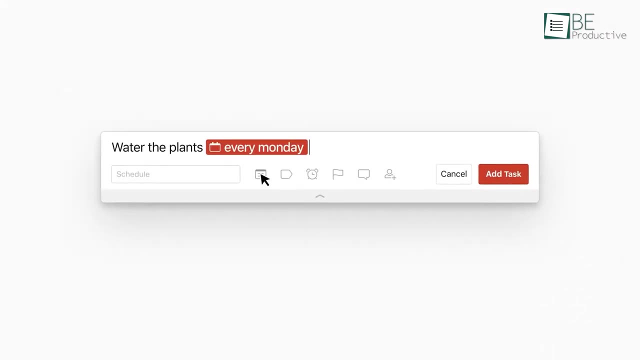 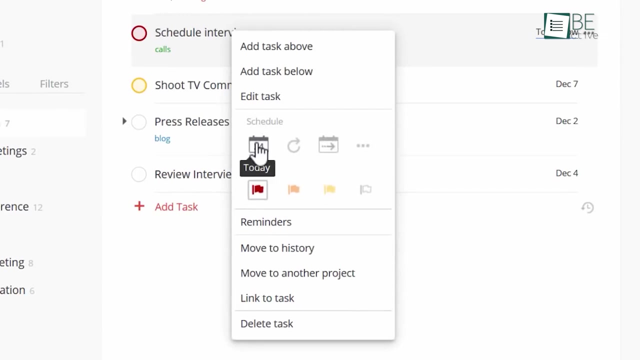 Runner up on the list is Todoist, an innovative task manager and do-list app that helps you effortlessly organize your task. With its user-friendly interface and natural language typing feature, you can create and manage tasks, prioritize and categorize them, set deadlines and reminders, and collaborate with others to achieve your goals. It also allows you to 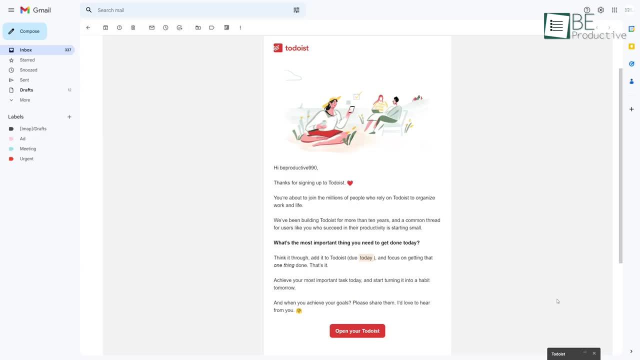 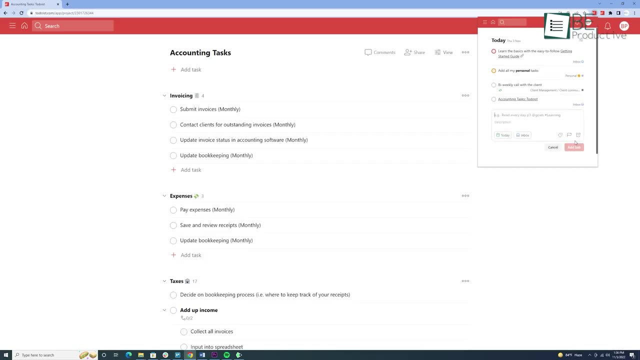 view all your tasks, create emails and allows cross-device syncing and cross-app integration, allowing you to convert your emails and slack messages into tasks across your computer and phone. With the Chrome extension, you can even add a browser link as a task. With its flexible project management and task viewing options, you can remain on top of. 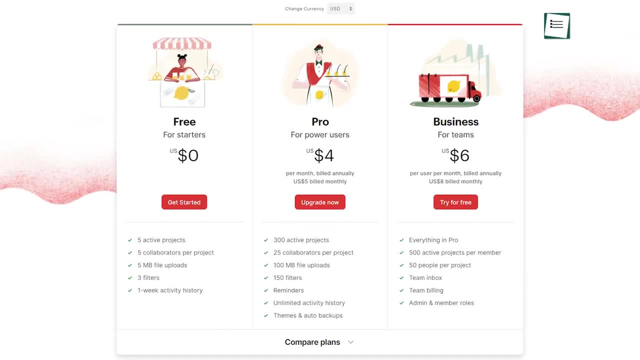 everything you need to do. It comes with plans for individuals and teams of all sizes. While you can access all these features for free, you can also upgrade to a premium plan for additional features, such as adding tasks based on location or adding tools that add additional. 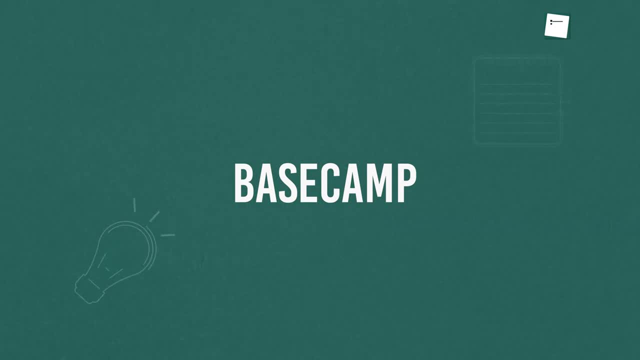 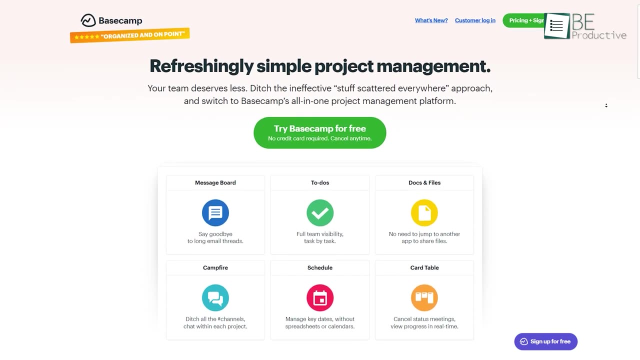 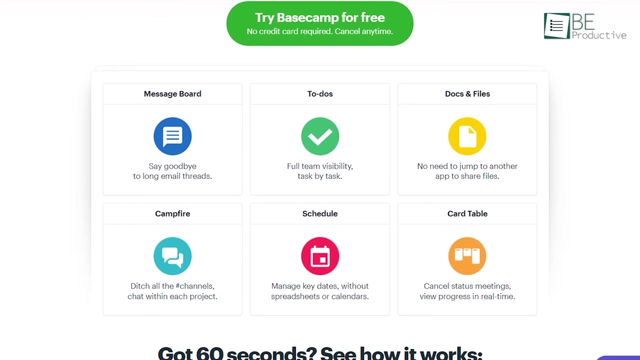 tags and labels. Next up is Basecamp, the ultimate task management tool that allows you to access essential features such as to-do lists, message boards, file sharing, chat rooms and calendars, to help teams stay organized and collaborate effectively With Basecamp's one-page. 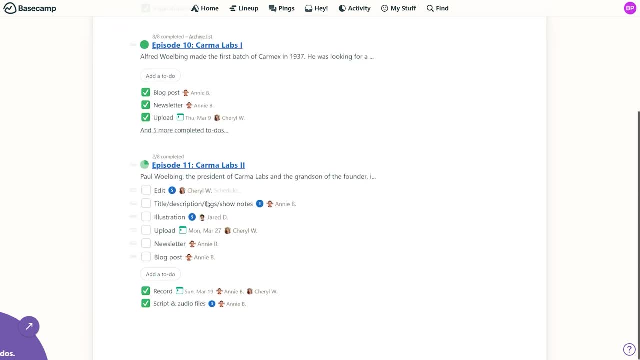 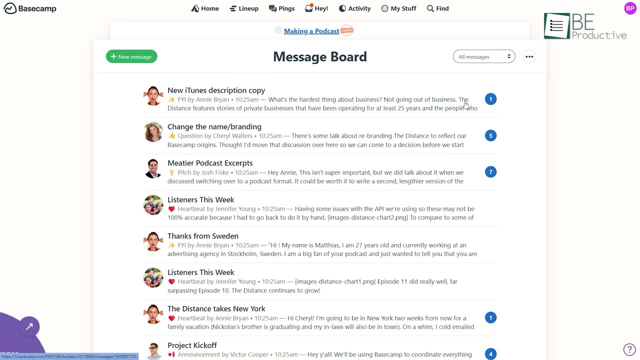 dashboard, centralized messages and powerful to-dos- to-do lists. from creating tasks and assigning tasks and deadlines to sharing announcements, updates, feedback and questions with your team or clients, you can do anything. Moreover, you can also store and organize files. 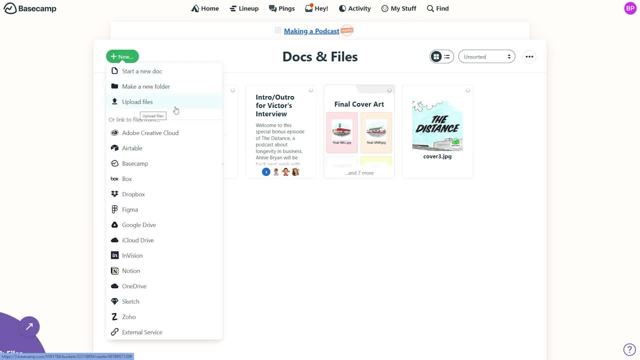 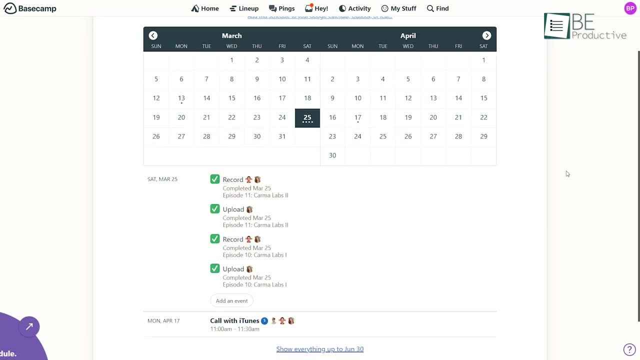 of any type and size with Basecamp's file sharing feature, and make real-time conversations with everyone with the chat room feature. While the calendar feature allows you to schedule events, meetings, milestones and deadlines, the door feature allows you to link other services like 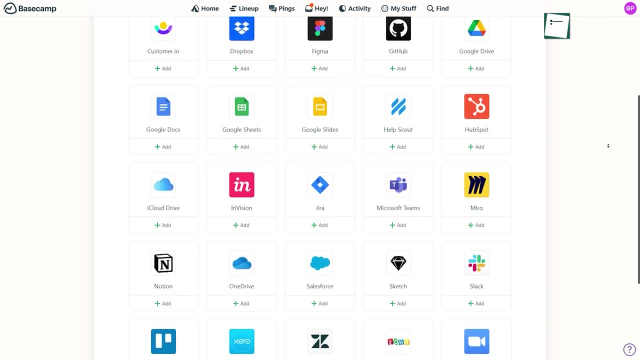 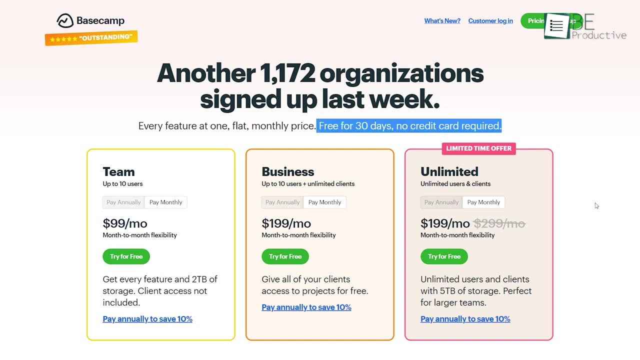 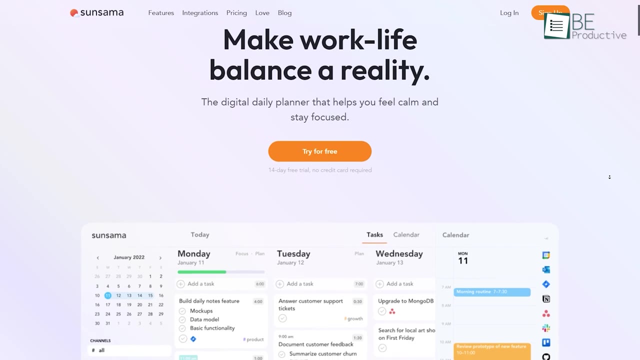 email, Google Drive, Dropbox, Zoom and Google Play Zoom and Slack to enhance your workflow. You can access all these features with a 30-day free trial and also upgrade to a paid plan for further use. Number 4 on the list is Sunsama, a powerful yet user-friendly task management software. 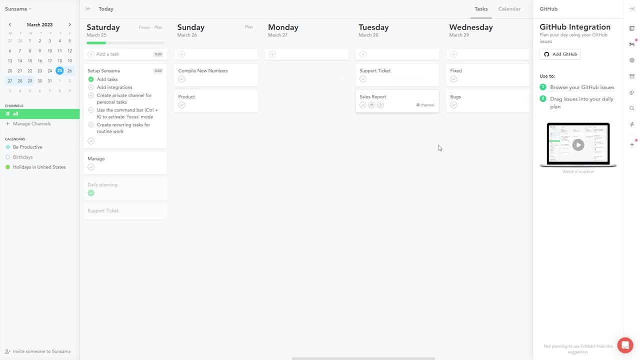 that provides a comprehensive view of your calendar and tasks in one place. It offers a daily planning ritual, timeboxing and sustainable work features to help you plan your day effectively. You can plan your day with the daily workflow that displays your task list and calendar side by: 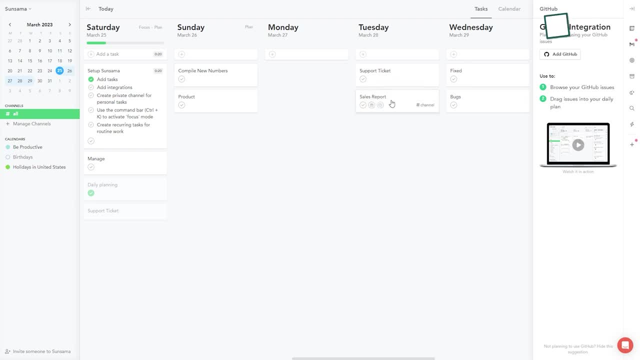 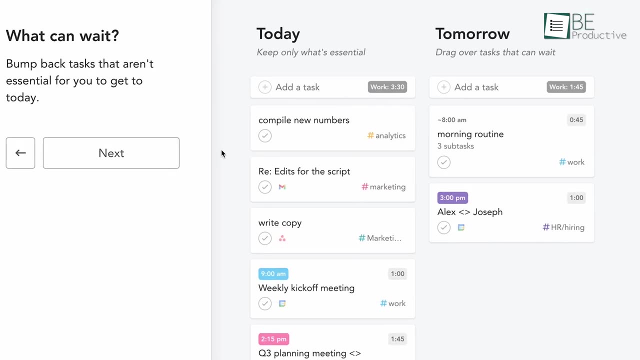 side. In addition, you can drag and drop tasks to schedule them on your calendar, add notes from meetings, set reminders, mark tasks as done and more. It also offers features like recurring tasks, task prioritization, subtasks and project management to help you stay organized. 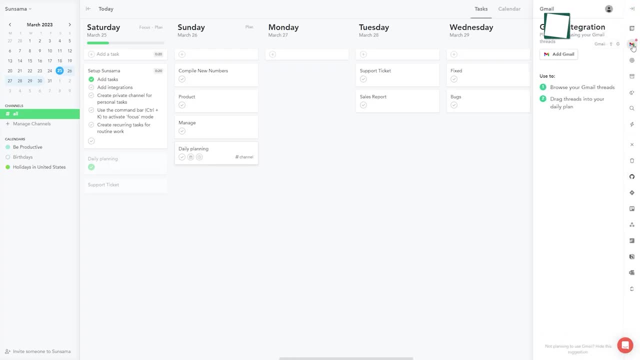 This innovative platform centralizes all your tasks in one place and avoids switching between multiple apps by allowing you to collect tasks and schedule them in one place. You can also collect tasks from various external tools, such as email, Asana, Trello, Gmail and Slack. 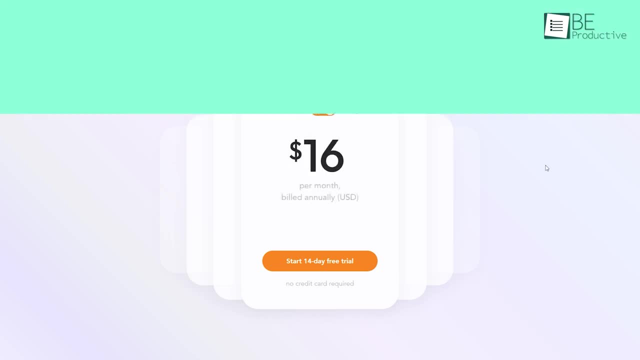 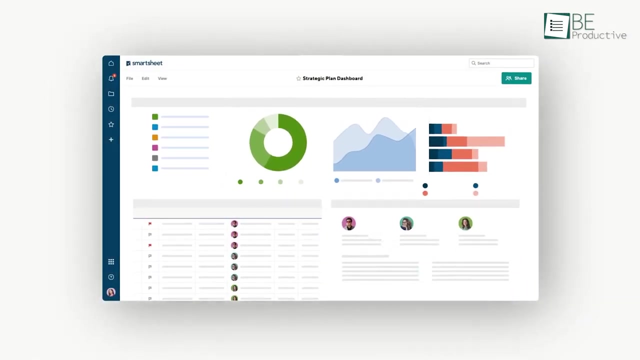 It comes with a premium plan along with a 14-day trial Coming up. we have Smartsheet, a collaborative task and project management platform that is designed to be flexible and customizable to meet your specific needs. This simple yet powerful task management platform adapts to your needs and helps you. 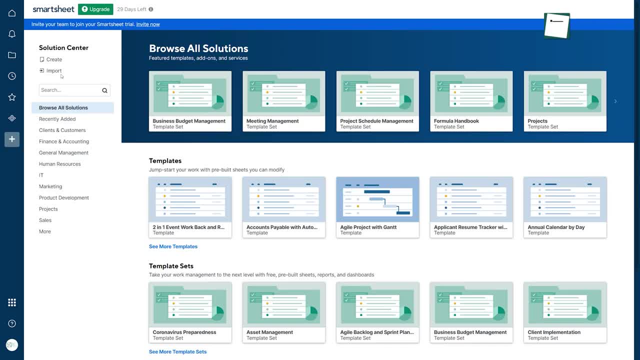 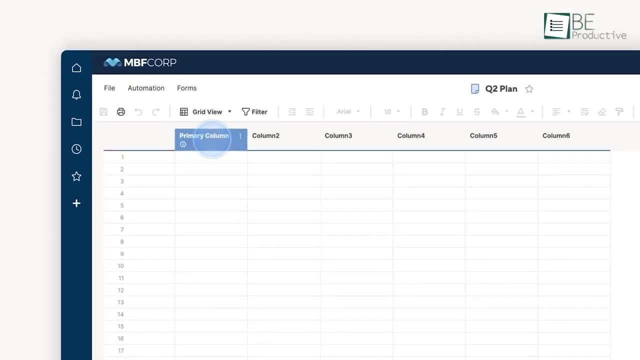 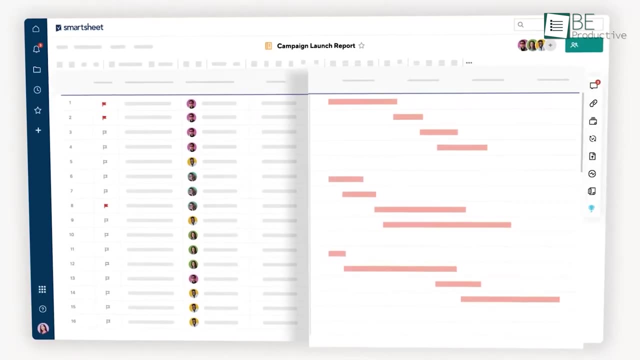 in achieving your goals. It allows you to create sheets for different types of tasks, like projects, budgets and inventories. You can also customize the sheets with columns, formulas, filters and attachments. With its variety of views, such as grid cart, Gantt chart and calendar, it allows you to create dashboards and reports for data. 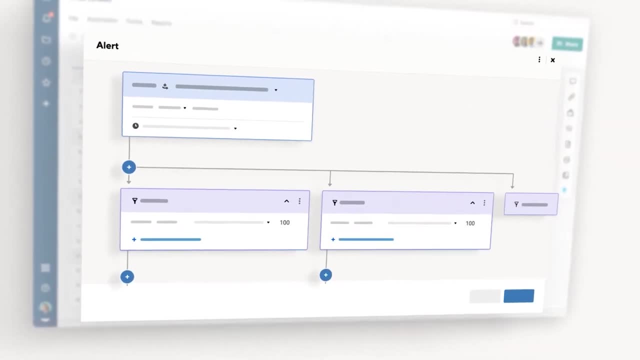 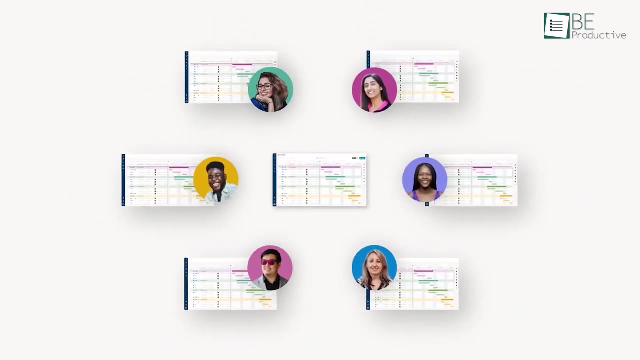 visualization and sharing. Moreover, it also enables the automation of workflows and processes with triggers, actions and forms. You can also facilitate collaboration through comments, mentions and feedback. You can also create a dashboard for different types of tasks, like and sharing of sheets, views and dashboards with different levels of access. 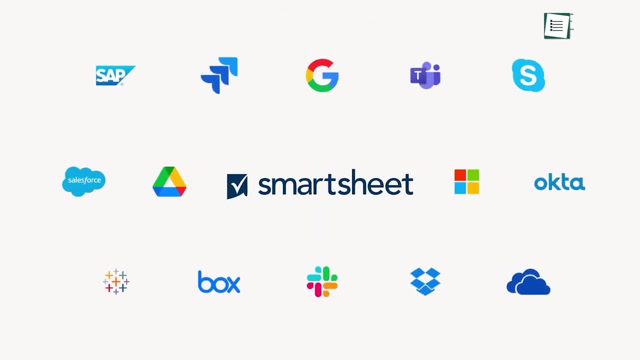 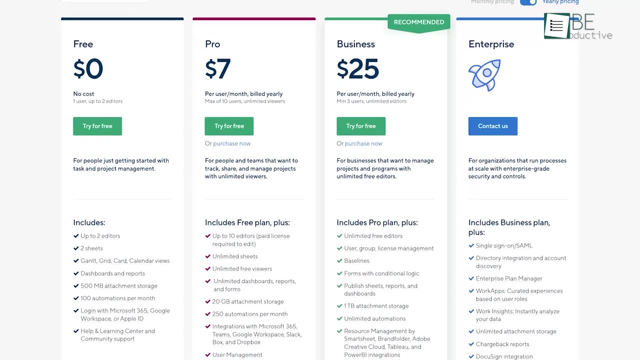 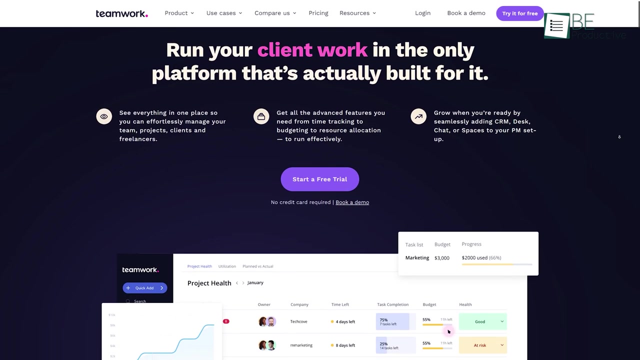 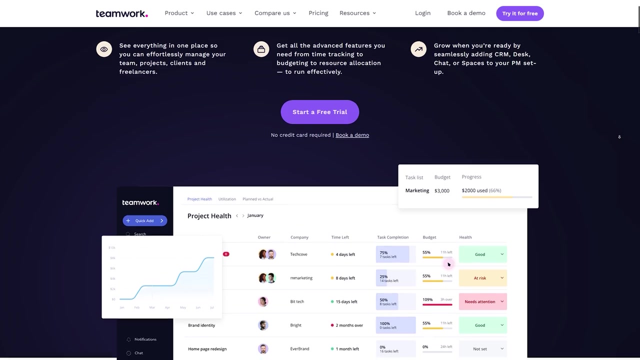 Furthermore, it can also integrate with popular tools like Microsoft 365 and Google Workspace. It comes with a forever free plan with limited features and different paid plans as well. Moving along the list, Teamwork is a task management software that fosters collaboration and timely project delivery for teams. With this software, 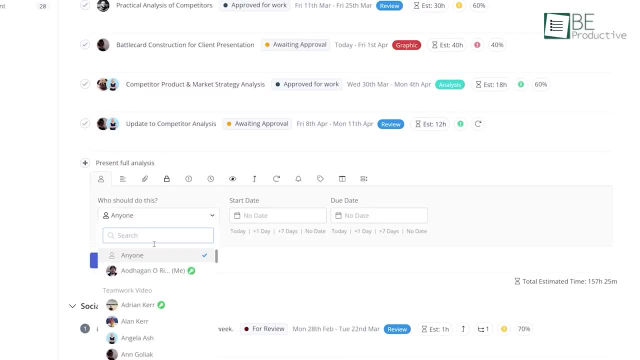 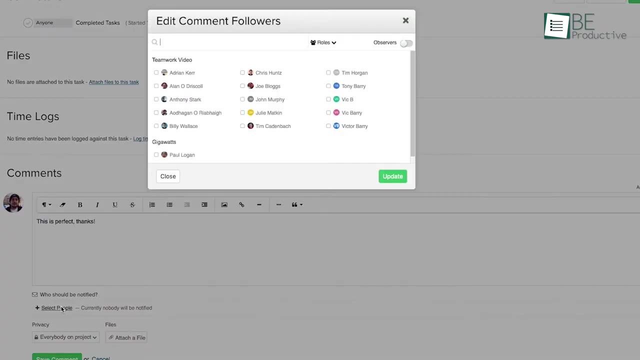 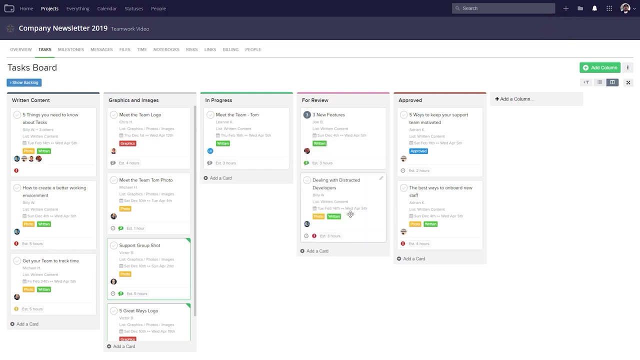 you can create tasks lists for each project and assign tasks to team members with due dates, priorities and dependencies. Moreover, you can also add comments, attachments, subtasks and tags to each task. The Kanban board view allows you to visualize tasks and drag and. 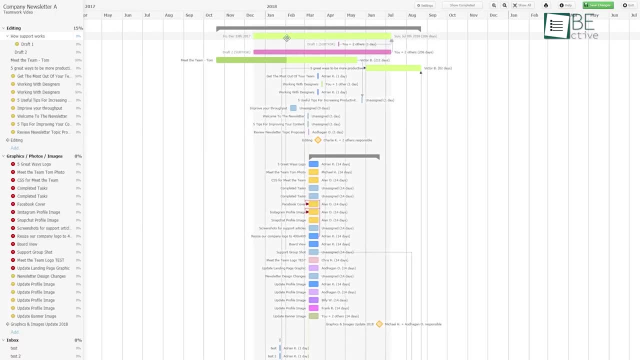 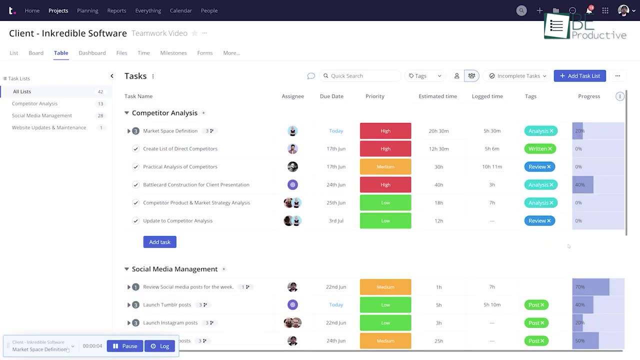 drop them across different stages as they progress. Apart from that, you can plan your projects with a Gantt chart and also log time spent on each task, manually or using a built-in timer with the time tracking feature. With the resource management tool, you can also manage your team's workload. 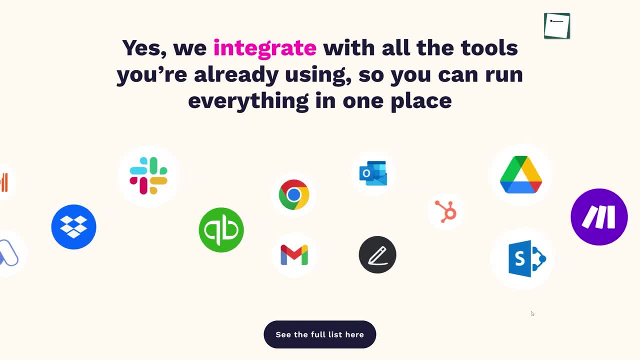 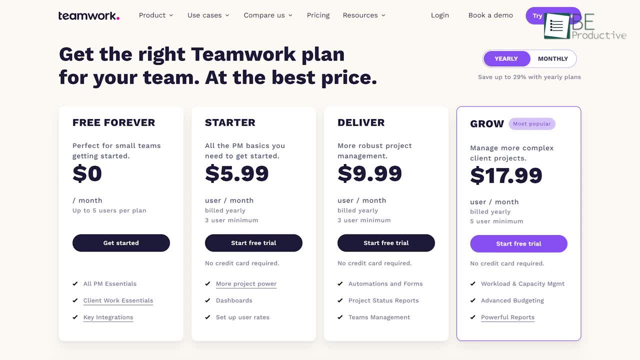 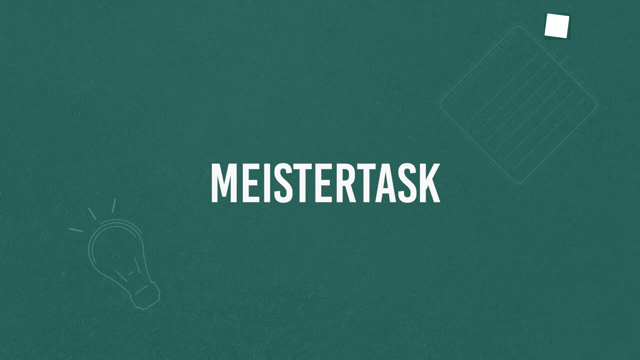 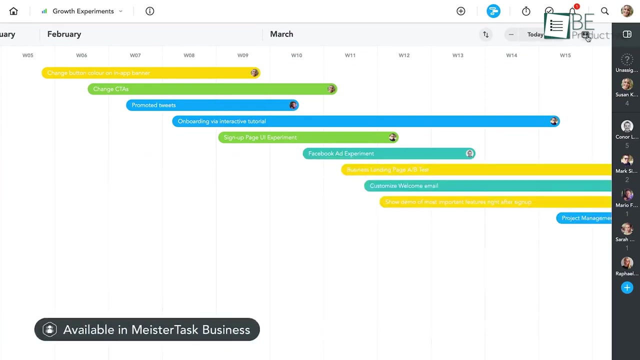 and availability. Additionally, it can integrate with popular tools such as Gmail, Outlook, Slack and Dropbox to streamline your workflow. You can access almost every feature with its forever free plan and upgrade to one of its paid plans anytime you want. Last software on our list is MeisterTask, a customizable task management software. 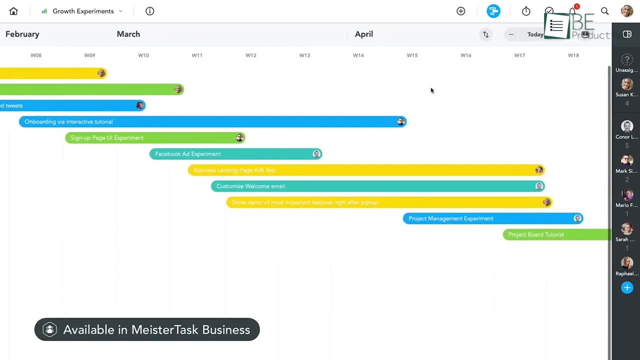 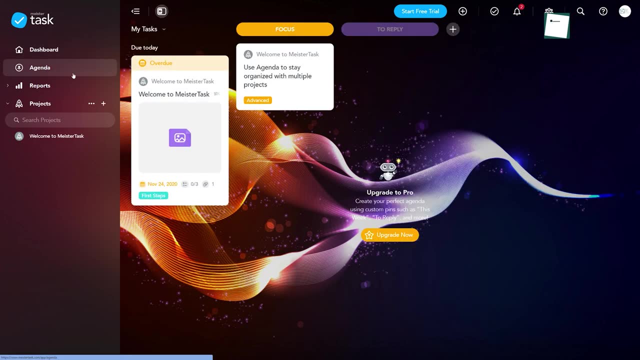 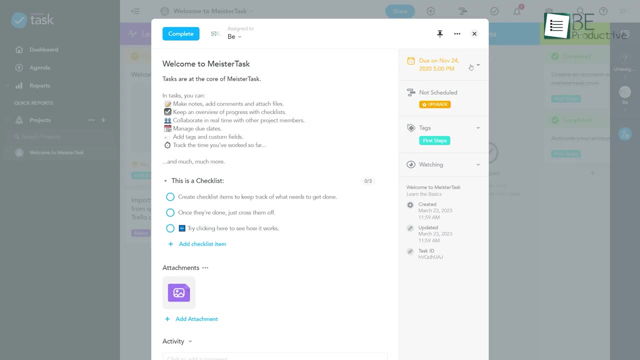 That helps teams stay organized and track progress from start to finish. The dashboard provides an overview of tasks and projects, including personal agendas, notifications, favorites and statistics, With its customizable project boards allowing users to create and assign tasks with due dates. 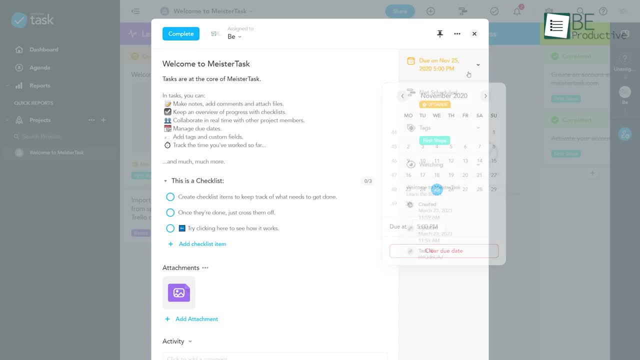 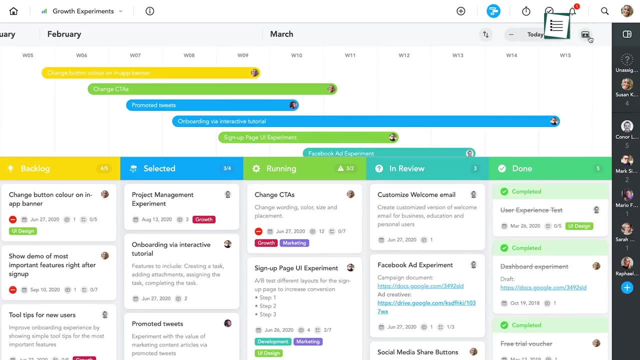 priorities, checklists, tags and attachments. While the Kanban-style project boards enable users to manage tasks and collaborate seamlessly, the Gantt-style timeline feature helps in assigning and scheduling tasks in calendar view, identifying bottlenecks and ensuring deadlines. 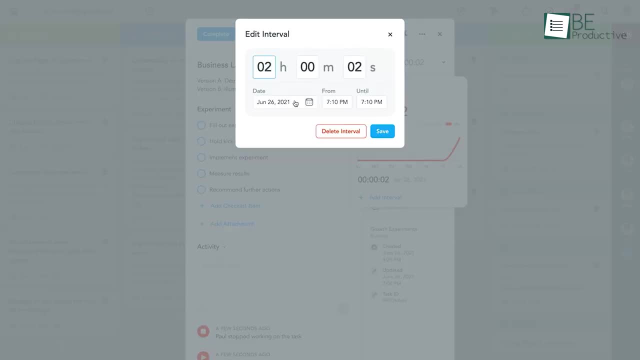 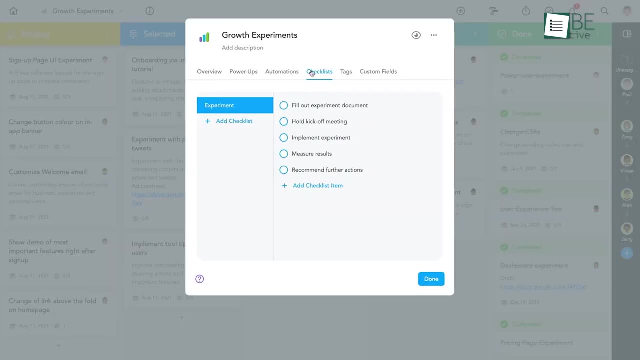 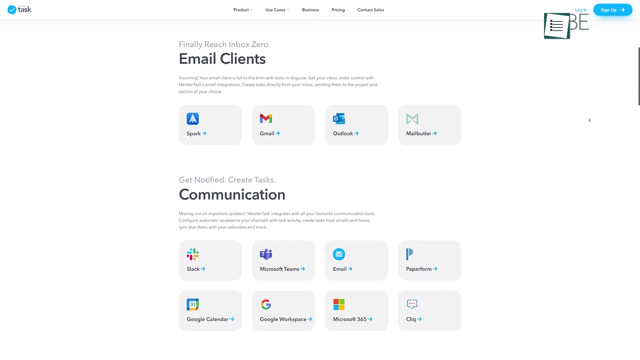 You can also track time with the built-in timer or with manual entries, and also enhance task descriptions with custom fields. Moreover, it also offers multiple checklist files and attachments, up to 200MB, integration with popular tools and task organization by tags. The free plan includes: 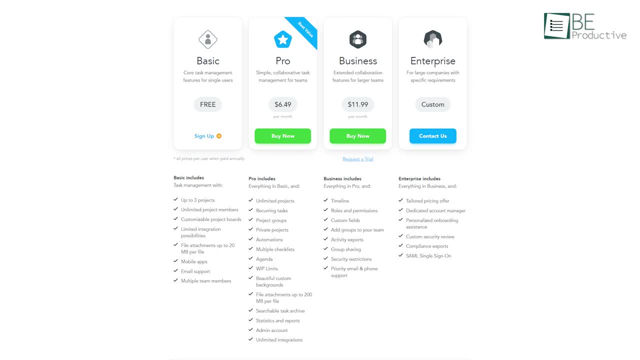 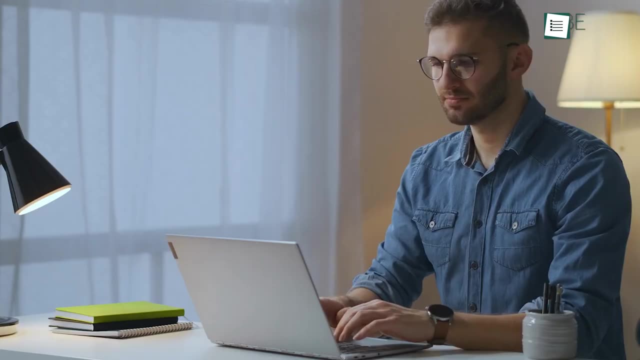 customizable project board for up to three projects and unlimited users and many more. For unlimited, unlimited projects and more features, you can also upgrade to any of its paid plans. So that was all about the 7 Best Task Management Softwares. Thanks for watching. If you found this video helpful, give it a thumbs up. 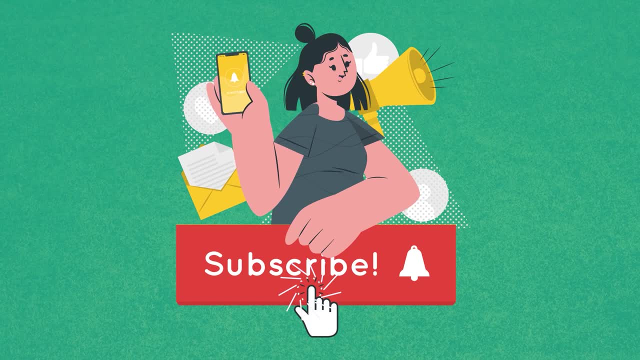 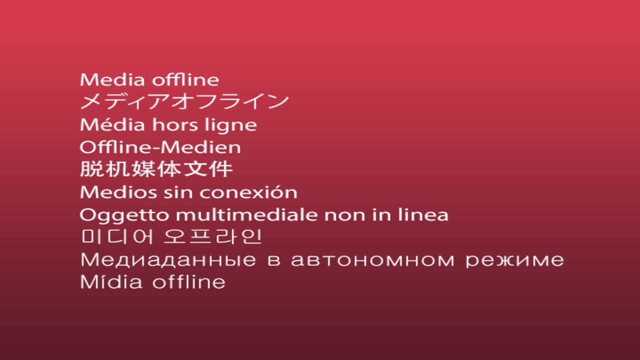 share it with your friends and let us know your thoughts in the comment section. Subscribe to our channel and hit the bell icon to see more videos like this on your feed. 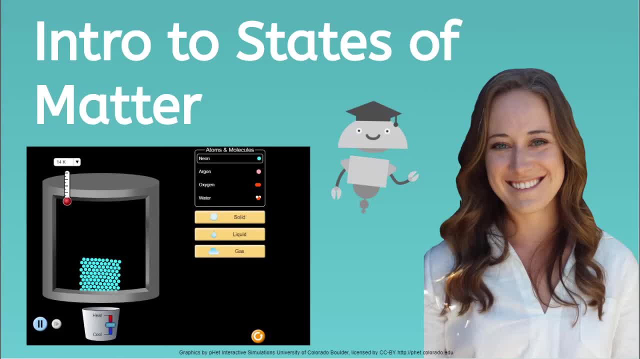 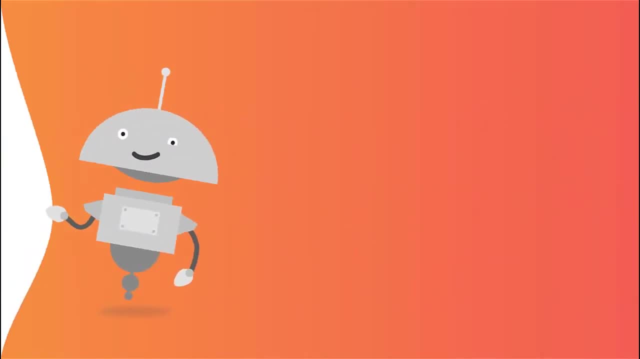 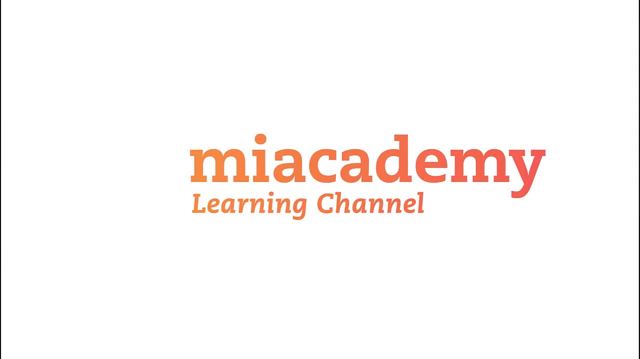 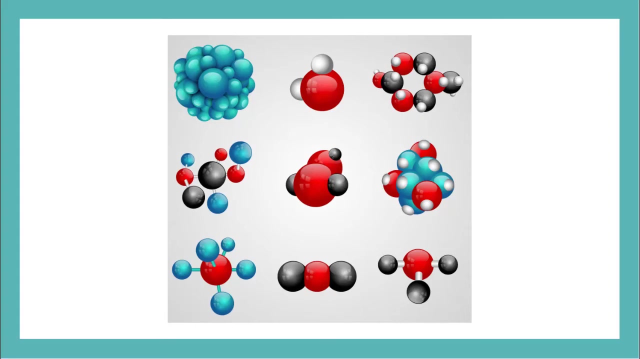 Hi there, my name is Kaylee and this lesson is all about the different states matter takes. Let's get going In the lesson. What is Matter? we learned that materials that are solids, liquids or gases are made out of matter, And matter is made up of tiny particles. 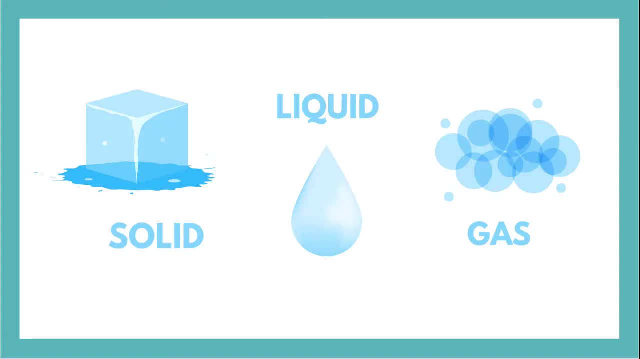 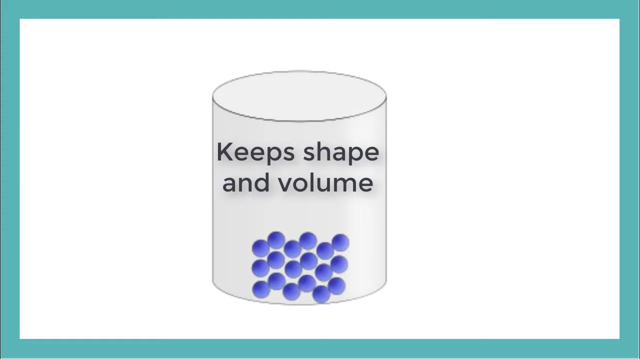 called atoms and molecules. Matter can exist in different states. We will study the main three: solid, liquid and gas. Solids are made up of matter with a specific shape and volume. We know there are solids because they hold their shape, regardless of what type of container we put them in. Solids act the way they do.